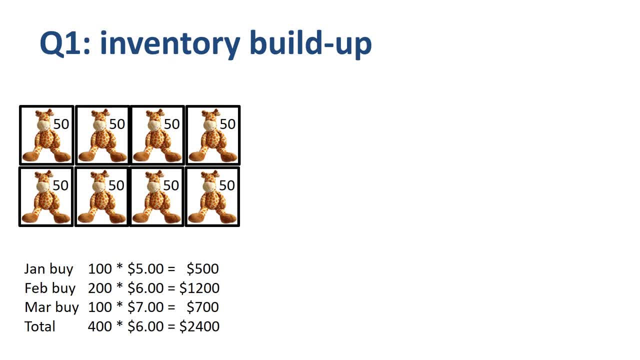 In the warehouse. the company does not specifically identify the boxes, they just stack them on a big pile For cost accounting and inventory valuation purposes. the company does keep track of the timing of the buys and the unit cost. Then we go to April. 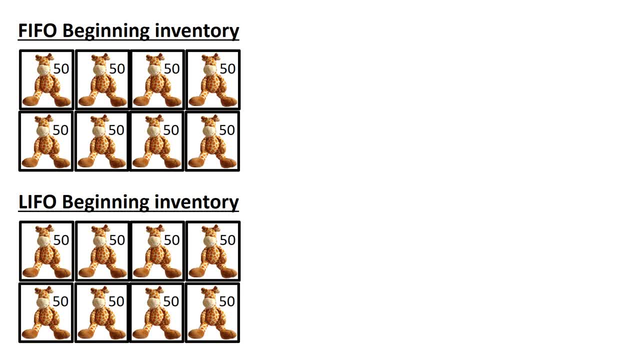 The ending inventory of Q1 is the beginning inventory of Q2.. The visual representation of the FIFO inventory flow is at the top. LIFO is at the bottom. The first box of Toy Giraffe's- 50 units, is sold in April. With FIFO first in, first out, we assume that the oldest inventory gets sold first. 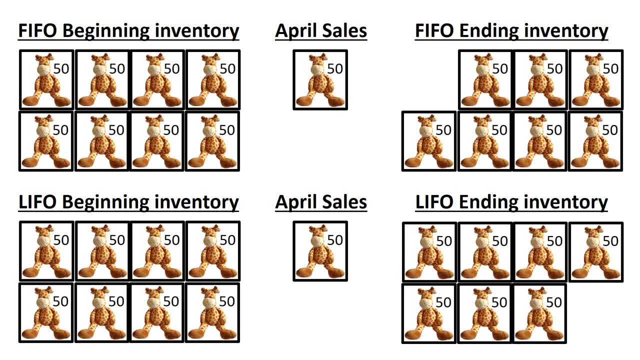 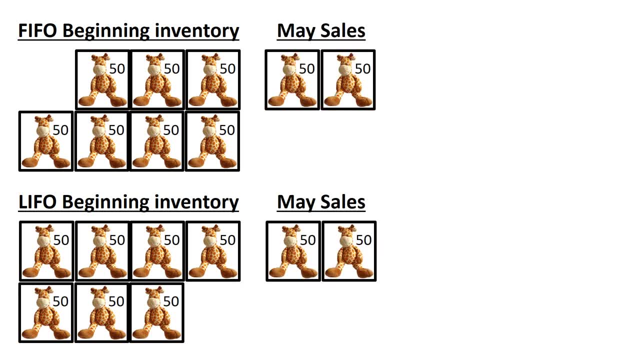 one of the boxes purchased in January With LIFO. last in, first out, we assume that the newest inventory gets sold first. one of the boxes purchased in March. Two boxes of Toy Giraffe's are sold in May With FIFO. first in, first out, we assume that the oldest inventory gets sold first. 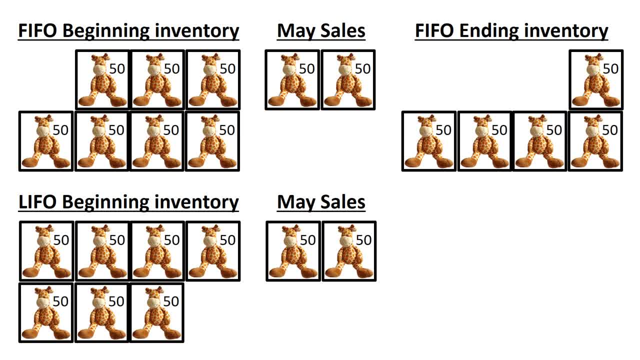 the last of the boxes purchased in January and one of the boxes bought in February. With LIFO, last in, first out, we assume that the newest inventory gets sold first, the last of the boxes purchased in March and one of the boxes bought in February. 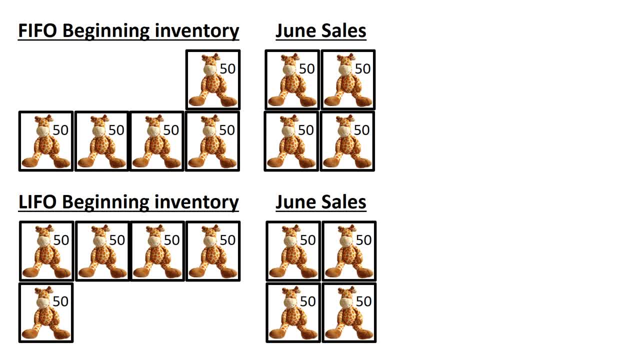 Four boxes of Toy Giraffe's are sold in June. With FIFO first in, first out. we assume that the oldest inventory gets sold first. the remaining three boxes bought in February and one box purchased in March. What stays in inventory at Q1 under FIFO is one box purchased in March. 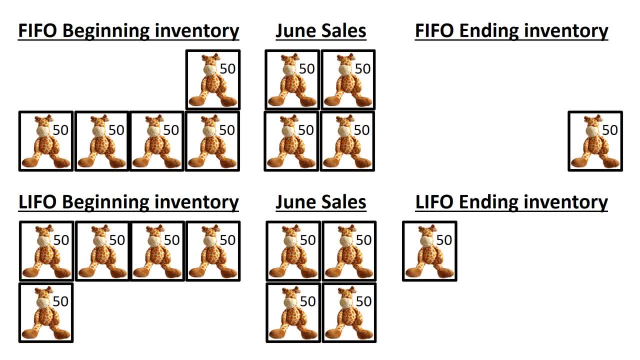 With LIFO last in first out. we assume that the newest inventory gets sold first. the remaining three boxes bought in February and one box purchased in January With LIFO last in first out. we assume that the newest inventory gets sold first. the 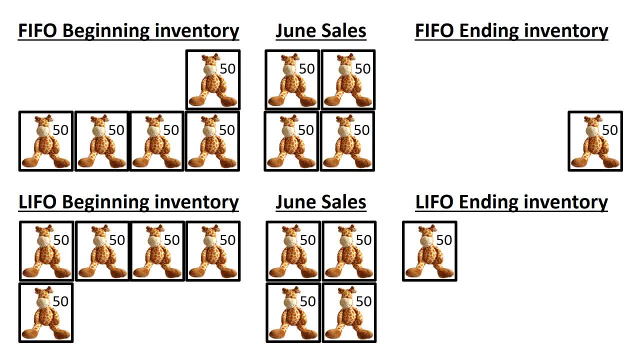 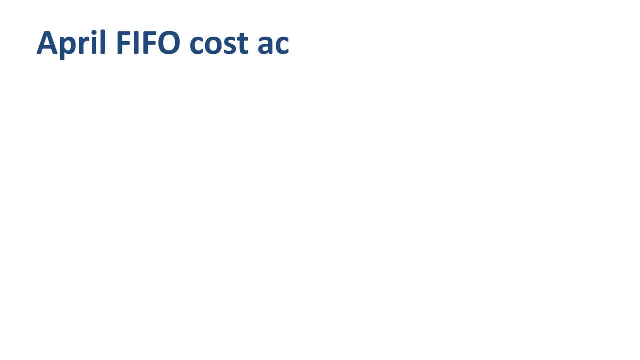 remaining three boxes bought in February and one box purchased in January. What stays in inventory at quarter end under LIFO is one box purchased in January. Let's compare FIFO and LIFO numerically. For both FIFO and LIFO, the number of units in inventory at both the start and the end. 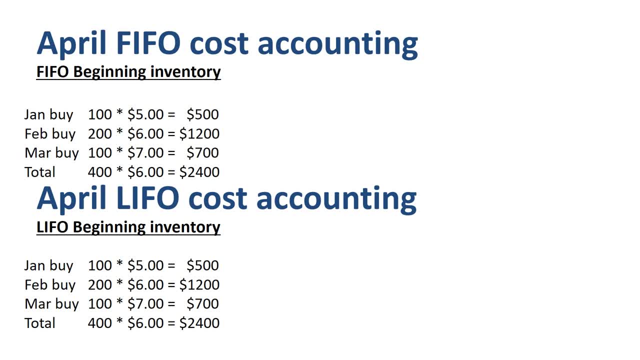 of April is the same. The ending inventory is 7 boxes of 50 units each, 350 units in total. For inventory valuation, as well as determining cost of goods sold, it is important to determine what is the cost per unit for this specific box. 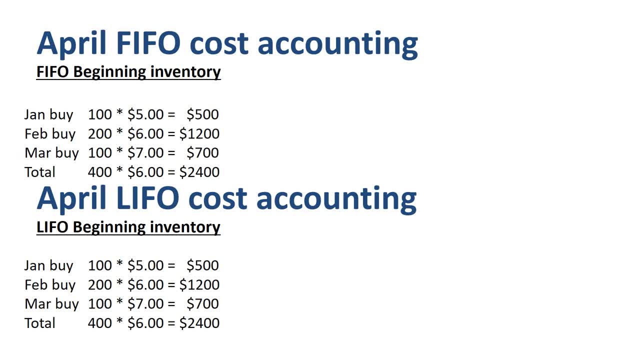 With FIFO first in, first out. we assume that the oldest inventory gets sold first. so we assume that the box sold originated from the January buy. What remains in inventory at the end of April is 50 units from the January buy, the full. 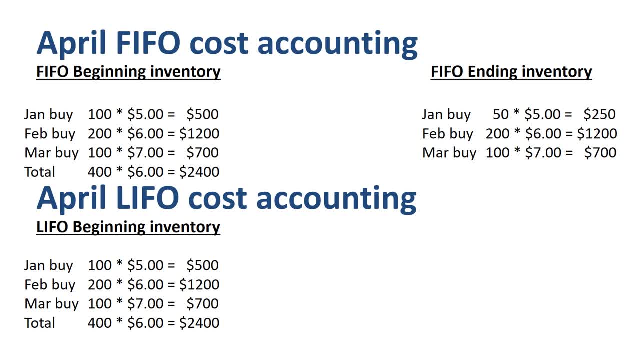 200 units from the February buy and the full 100 units from the March buy. In total 350 units with a total purchase price of $2,150.. So on average $6.14 per unit, an increase of the weighted average unit cost up from. 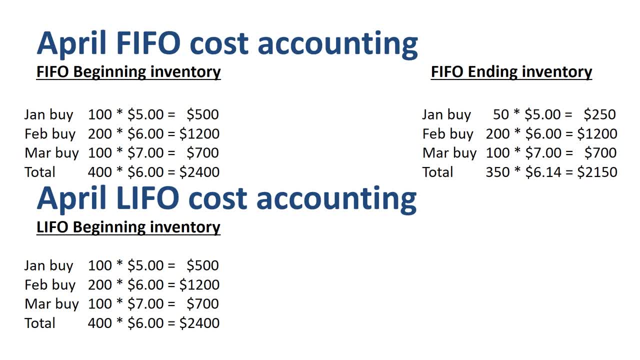 $6 previously. If we prepare the income statement for April, revenue is 50 units times $10 is $500,. cost of goods sold, or COGS, is 50 units times $5 is $250, and gross profit is $250.. Out of the January buy that was part of the beginning inventory, 50 units go to COGS and 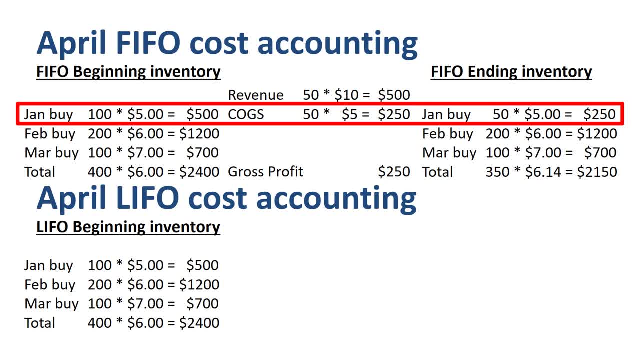 50 units go to the end of April. With FIFO first in, first out, we assume that the oldest inventory gets sold first. so we assume that the box sold originated from the March buy. What remains in inventory at the end of April is the full 100 units from the January buy. 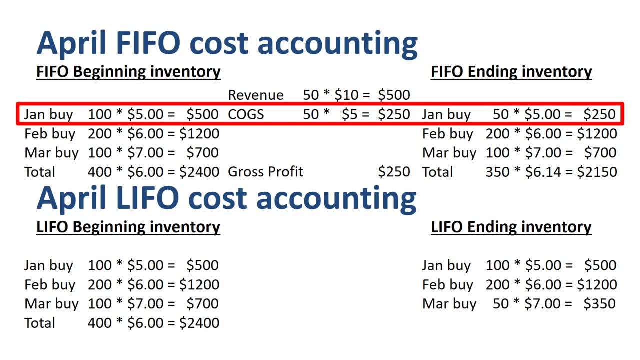 the full 200 units from the February buy and the remaining 50 units from the March buy. In total 350 units with a total purchase price of $2,050.. So on average $5.86 per unit. That's the end of April. 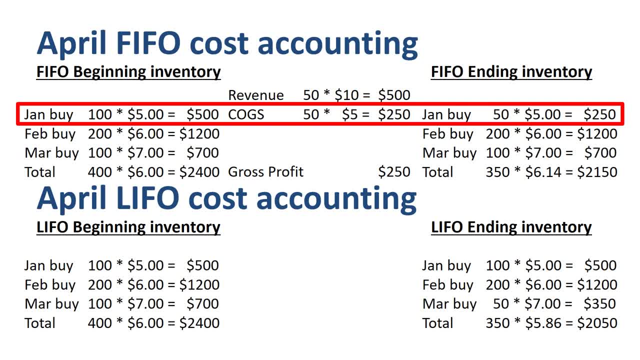 If we prepare the income statement for April, revenue is: 50 units times $10 is $500, cost of goods sold, or COGS, is 50 units times $7 is $350, and gross profit is $150.. Out of the March buy that was part of the beginning inventory, 50 units go to COGS and 50 units 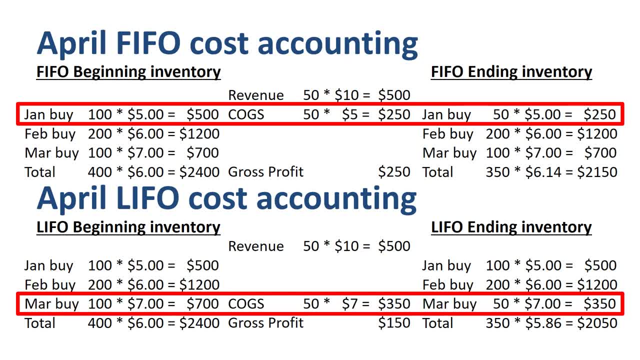 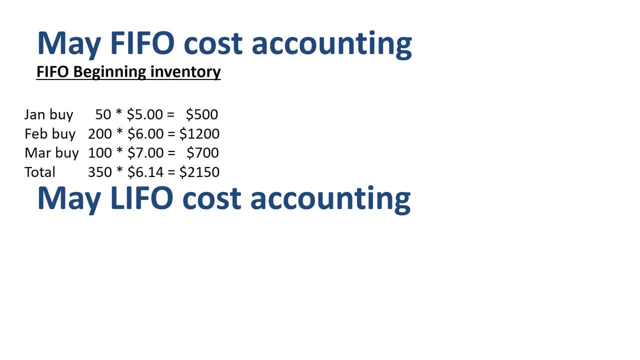 go to the ending inventory Onward to May. The ending inventory is 5 boxes of 50 units each, 250 units in total Applying FIFO. what remains in inventory at the end of May is 0 units from the January buy, 150 units from the February buy and the full 100 units from the March buy. 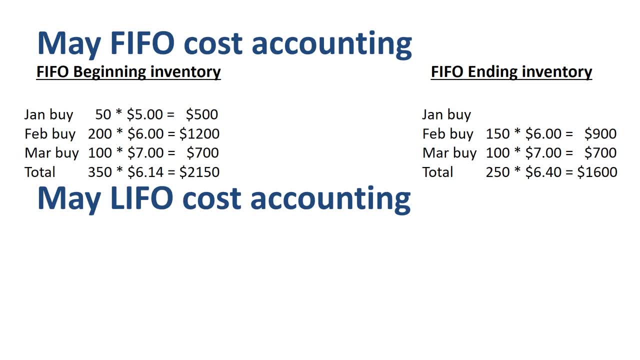 In total 250 units with a total purchase price of $1,600.. So on average $6.40 per unit. If we prepare the income statement for May, revenue is 100 units times $10 is $1,000, cost: 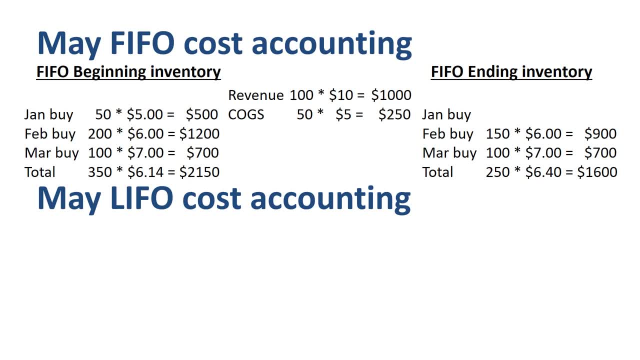 of goods sold, or COGS, is 50 units times $5, is $250, plus 50 units times $6 is $300, and gross profit is $450.. Out of the remaining January buy, that was part of the beginning inventory. we took all. 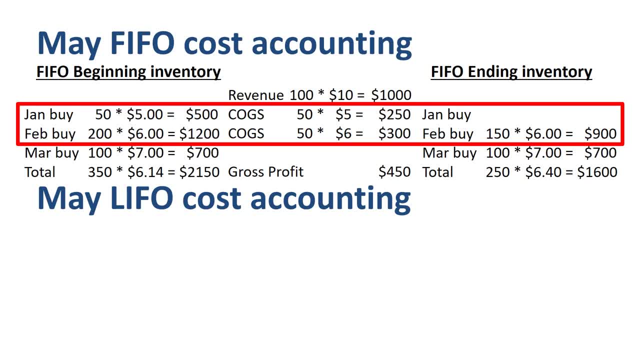 50 units to COGS and we took 50 units from the February buy into COGS. The remaining 150 units from the February buy go to the ending inventory Applying LIFO. what remains in inventory at the end of May is the full 100 units from. 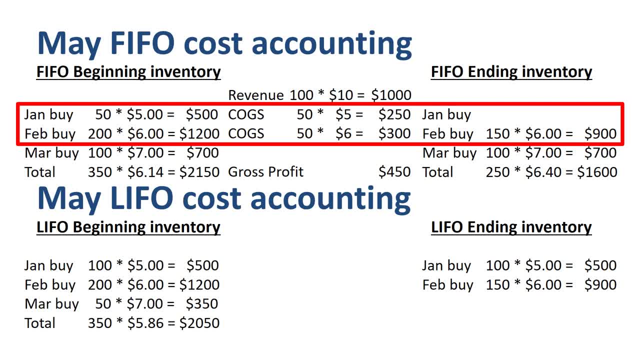 the January buy 150 units from the February buy and no units from the March buy. In total 250 units with a total purchase price of $1,400. So on average $5.60 per unit. If we prepare the income statement for May, revenue is 100 units times $10 is $1,000,. 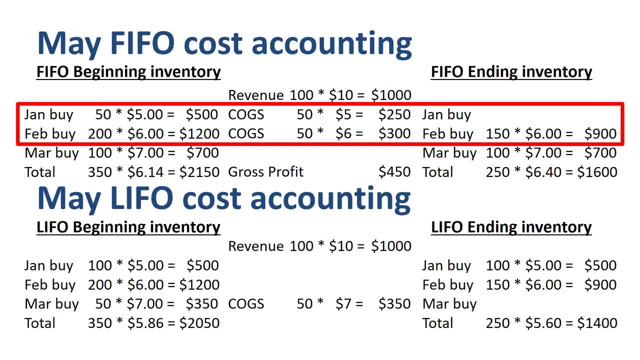 and gross profit is $1,000.. Cost of goods sold, or COGS, is 50 units times $7, is $350, plus 50 units times $6 is $300, and gross profit is $350.. Out of the remaining March buy, that was part of the beginning inventory. we took all 50. 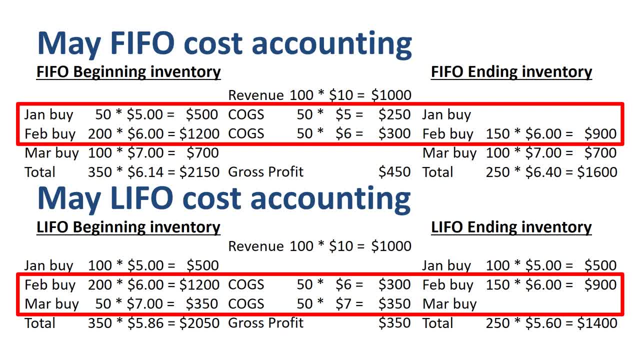 units to COGS and we took 50 units from the February buy into COGS. The remaining 150 units from the February buy go to the ending inventory Onward to June. The ending inventory is just one box of 50 units. 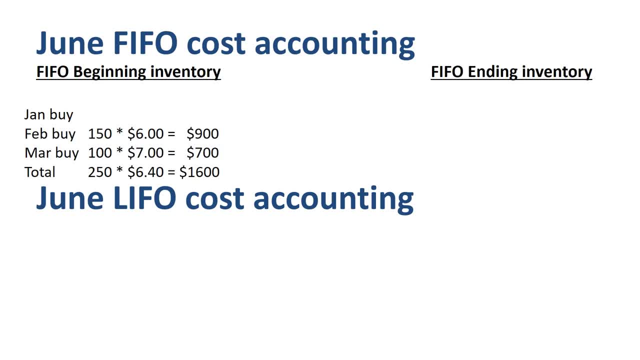 Applying FIFO. what remains in inventory at the end of June is just 50 units from the March. buy 50 units of $7 each. $350. in total, If we prepare the income statement for June, revenue is 200 units times $10 is $2,000,. 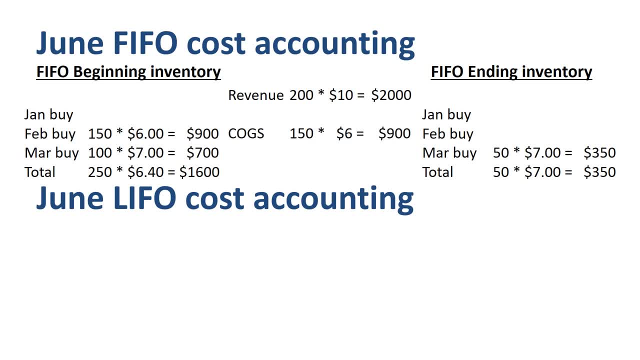 cost of goods sold, or COGS, is 150 units times $6 is $900, plus 50 units times $6 is $800, and gross profit is $2,000.. If we prepare the income statement for June, revenue is 200 units times $10 is $2,000, and 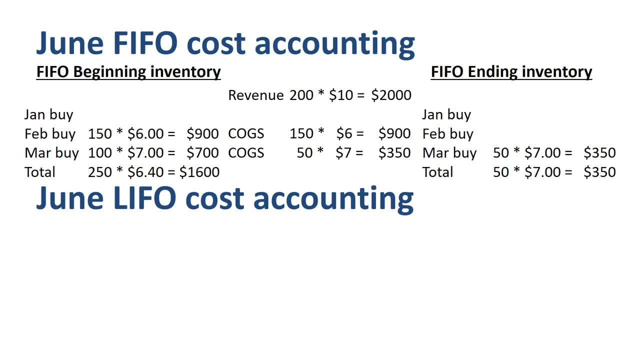 this time $7 is $350, so total COGS of $1,250, and therefore a gross profit of $750.. Out of the remaining February buy, that was part of the beginning inventory. we took all 150 units to COGS and we took 50 units from the March buy into COGS. 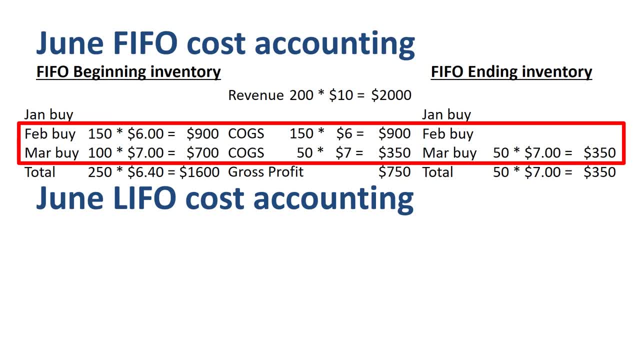 The remaining 50 units from the March buy go to the ending inventory. Applying LIFO: what remains in inventory at the end of June is just 50 units from the March buy into COGS. The remaining 50 units from the March buy go to the ending inventory. 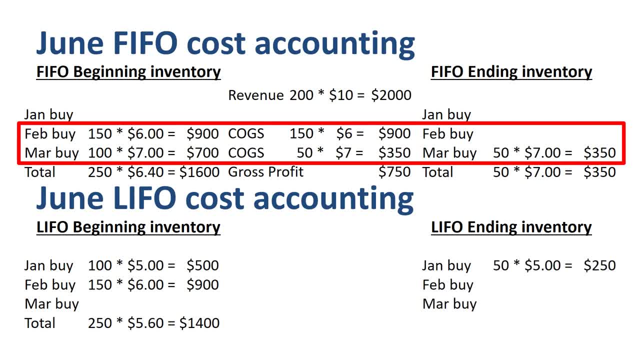 If we prepare the income statement for June, revenue is: 200 units times $10 is $2,000,. cost of goods sold, or COGS, is 150 units times $6 is $900, plus 50 units times $5 is $250,. so 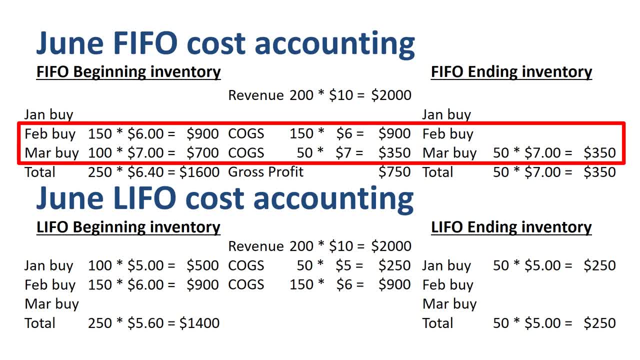 total COGS of $1,150, and therefore a gross profit of $850.. Out of the remaining February buy, that was part of the beginning inventory. we took all 150 units to COGS and we took 50 units from the January buy into COGS. 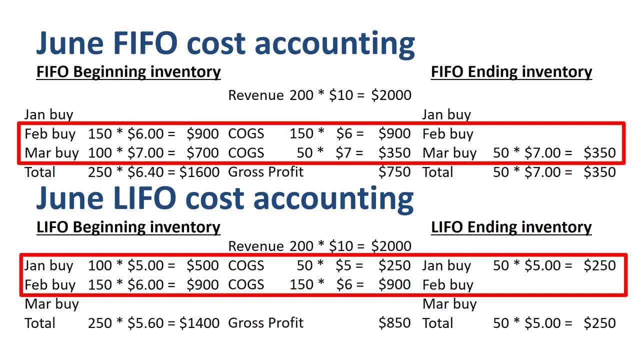 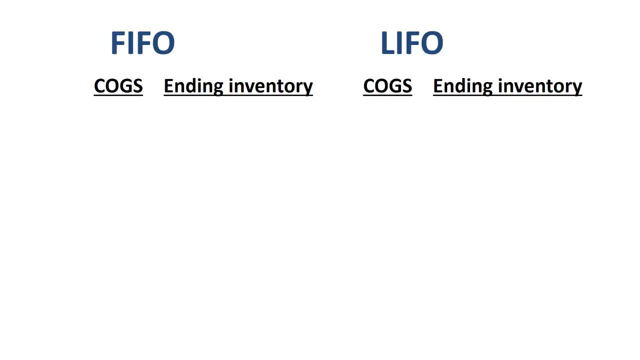 The remaining 50 units from the January buy go to the ending inventory. To summarize FIFO versus LIFO, here are the cost of goods sold and ending inventory values by period. With FIFO first in, first out, We assume that the oldest inventory gets sold first. 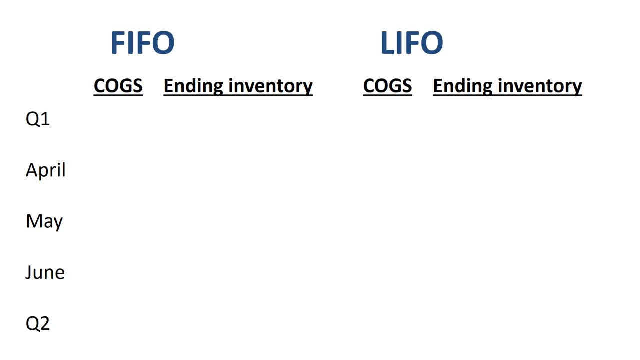 With LIFO. last in, first out. we assume that the newest inventory gets sold first In both the FIFO and the LIFO method. no COGS in Q1, as we did not sell anything. FIFO cost of goods sold: $250 in April, $550 in May, $1,250 in June, $2,050 for all of Q2.. 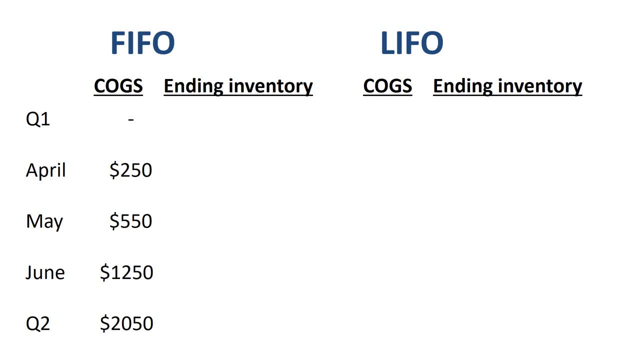 The ending inventory value is simply the previous period's inventory value and the ending value is the $550.. period's inventory value minus this month's COGS Start with $2400 at the end of Q1, then $2150 end of April. $1600 end of May, $350 for end.